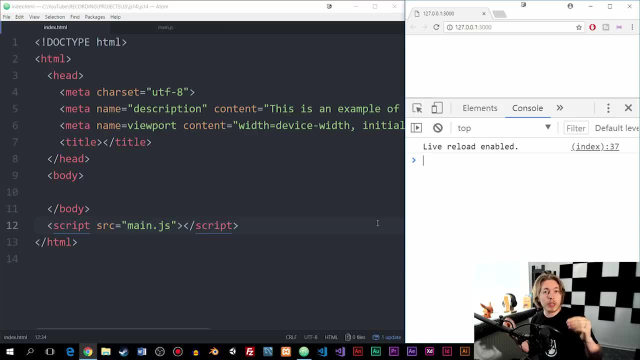 And it's something we use in order to easier structure our code or reuse code later on inside our scripts. So, when it comes to these functions, we have two different reasons for using them. The first one is that we want to create a result immediately inside our code. 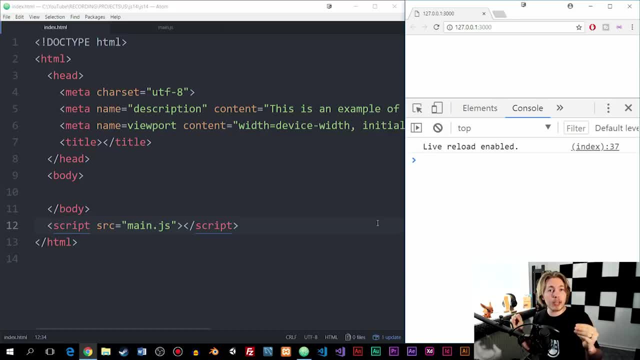 or we want to create an answer for other functions to use inside our JavaScript. So, when it comes to these functions, we have three different types. We have something called the name function, which is what we're going to mainly use here at the beginning of this course. 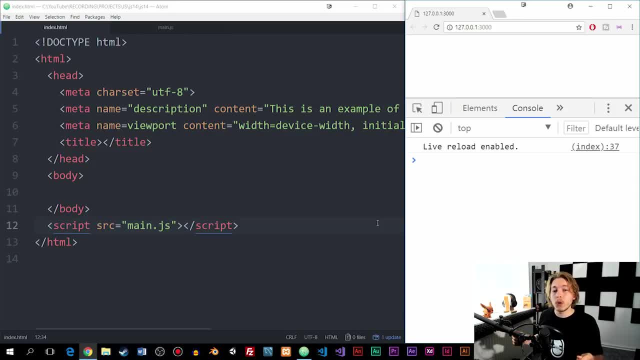 We have something called an anonymous function And then we have something called a immediately invoked functional expression, which is quite a fancy way of saying the name of a function. But there's some key differences between these three functions which we're going to go over. 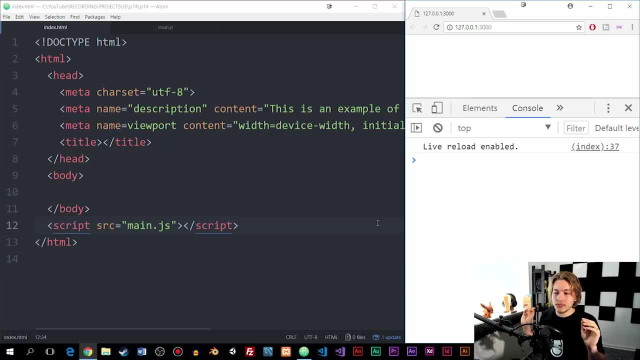 in this episode. So when it comes to these functions, I'm going to go ahead and take them one by one. As you can see in front of me, I do have a basic index page inside my website. here Now, I just want to point out that in this lesson here, I will be using an external file instead of 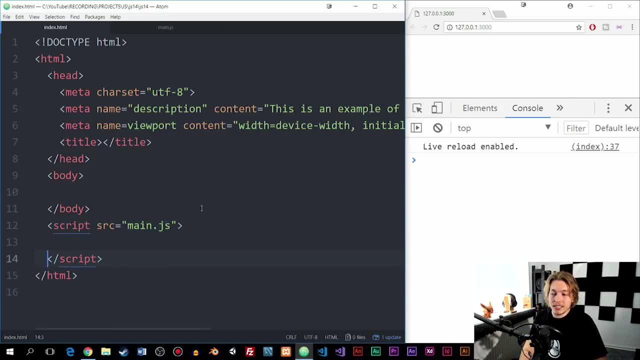 what we usually do by writing the JavaScript code directly inside the index page, by writing it in between the script tags. So this is going to be the first episode where we do actually use an external file by simply linking to it inside our index page. So whenever I write JavaScript, 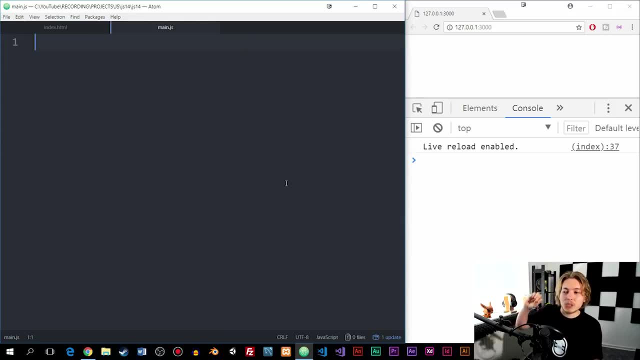 inside this mainjs. it's going to do the exact same thing as writing it inside the index page, just so you're aware of it. So the first example I want to create for you is something called a named function. Now, a named function we create by writing the function declaration. Then we create: 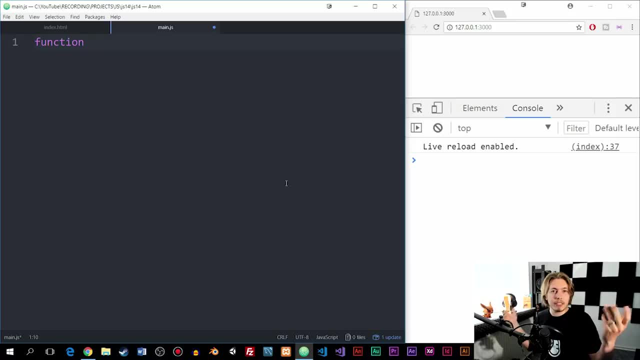 some kind of name for it, just like we do with variables, We can think of anything, So I'll just call it test example. Do you notice that when we use multiple words, it's a common habit inside programming: The words coming after the first word are going to start with a capitalized letter. So in this case, 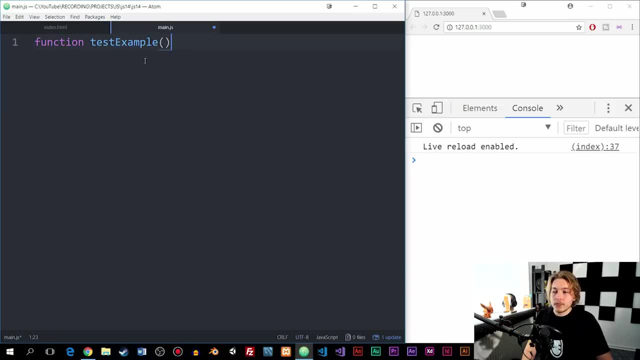 the E for the second word is going to be capitalized. So after the name we write parentheses, then we write curly brackets, and then we open and close the curly brackets, Then whatever goes in between this block of code, which is whatever's inside the curly brackets, 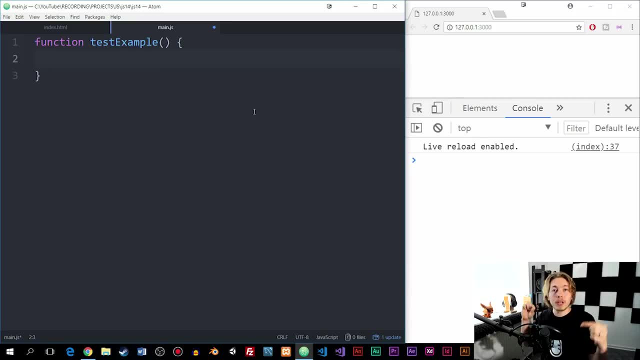 is going to be the code that is going to execute once I call on this function. here. The code that we can write in between the curly brackets can be anything from mathematical equations to just generating a random string or something. So in this case, I'm just going to go ahead and create. 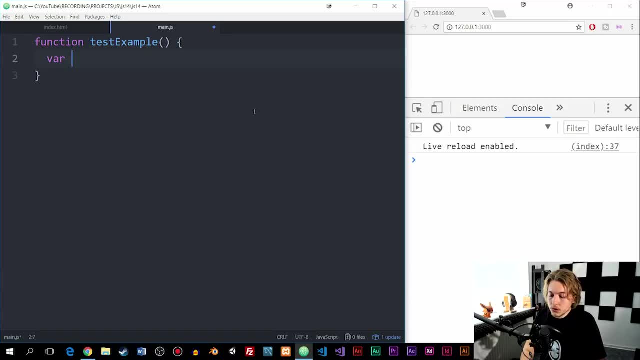 a variable which is going to be called greeting. I'm going to set it equal to hi. my name is Daniel. If I can actually spell my own name, there we go. Then afterwards, what I want to do is I want to actually get some kind of result from it. Now we can, if we want, to go ahead and write a. 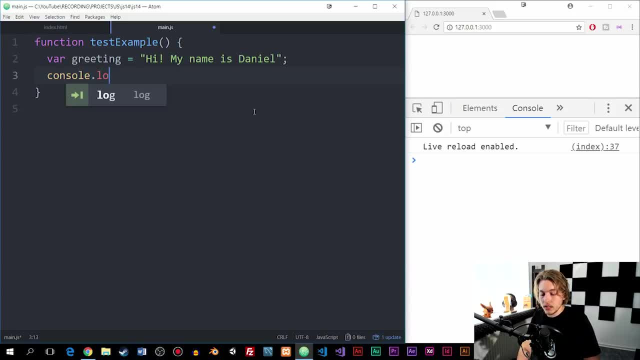 consolelog- consolelog and then simply consolelog out greeting, which is the variable up here. We will then say inside the console: hi, my name is Daniel. So what we basically created here is a block of code that doesn't actually run inside the website until we actually call. 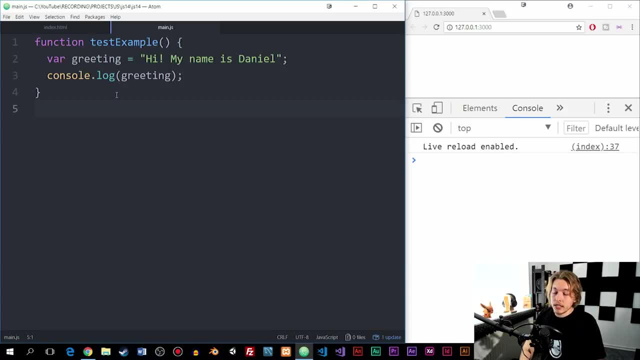 on the function inside our JavaScript. So what we can do to call it is we can go down to the next line here and say we want to run the actual function called test. example- Parentheses, semicolon- And then if we were to look inside the console, you can now see it says: 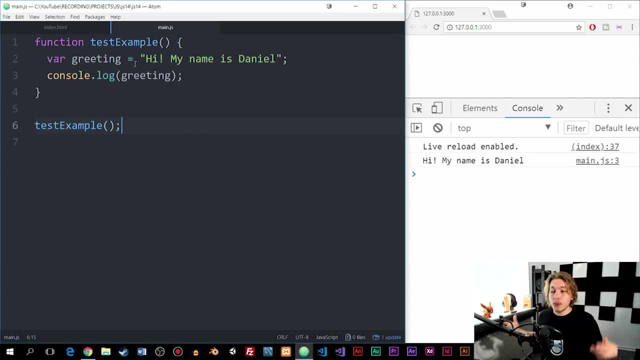 hi, my name is Daniel because I'm now running the function. Now, an important thing to mention about these named functions is that we can actually create them any place inside the code we want, and then we can use them any place inside our JavaScript code, So you don't need to place. 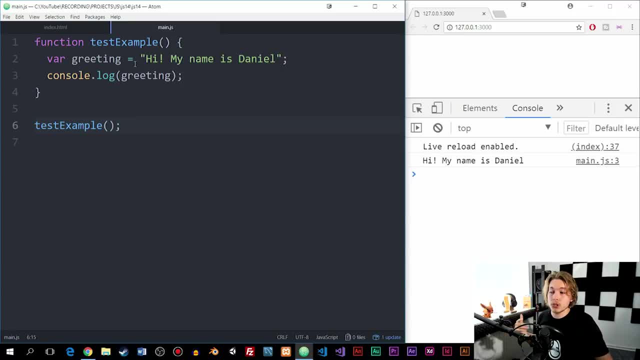 it a specific place for it to work inside the JavaScript when we want to call on it down here where it says, for example, test example. So the function could be either at the top or I could place it below test example, and it's still going to work inside the browser. So the 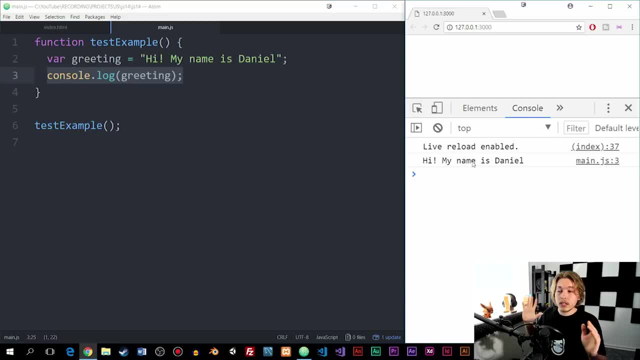 order doesn't really matter when we create these named functions here. Now, when it comes to functions, we usually do it in a slightly different way, because, instead of directly outputting anything from inside a function, we can also go ahead and return a value using the. 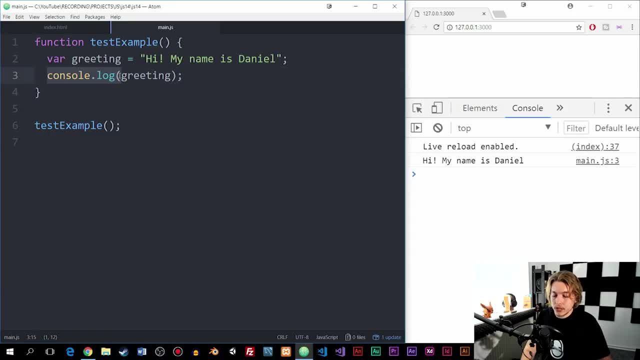 function. So instead of console logging it, instead we can actually go ahead and return some kind of result. So instead I'm returning greeting and as you can see, right now it doesn't actually say anything inside the browser here. But instead 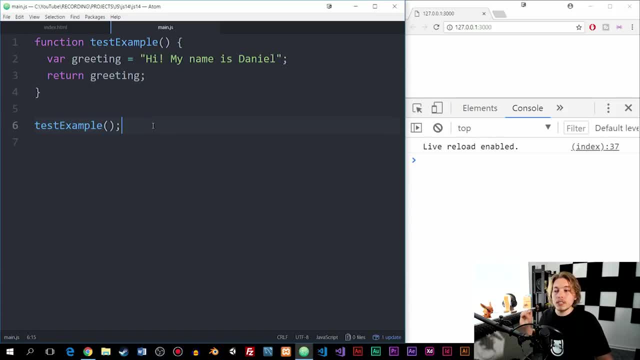 what we do is that when we call the function down here, we still have the result, which is: hi, my name is Daniel, but we stored it. we haven't actually outputted it yet. If I want to output the result from inside the function, the way we usually do it- is by going down where it did. 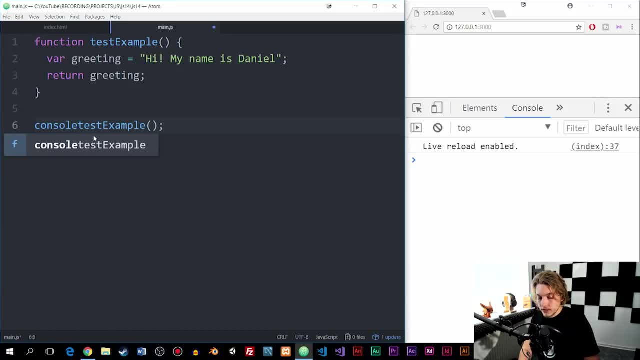 actually call in the function and console log it from down here instead. So I'm actually going to console log the entire function And, as you can see, I'm actually going to console log it from down here instead. So I'm actually going to console log the entire function And, as you can, 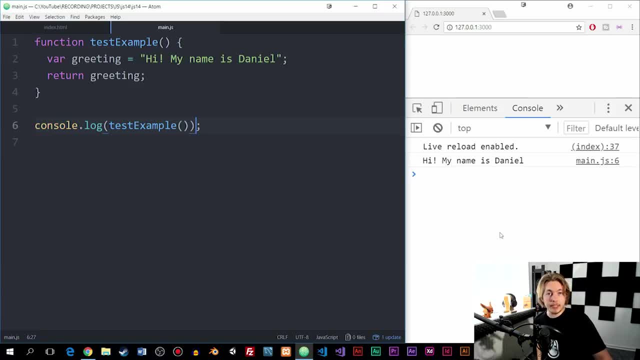 see inside the browser, here inside the console, we get: Hi, my name is Dan. Now, the last thing I want to show regarding name functions is that we can actually pass in parameters from outside the function and into the function So we can use it inside the function code. So in this example, 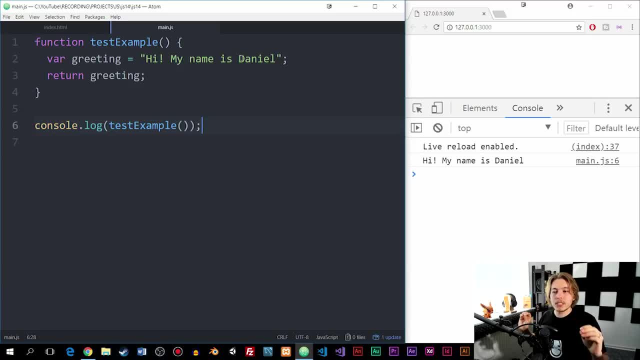 you can actually see we wrote. Hi. my name is Daniel, But what if I want to submit an actual name into the function instead of just having this default Daniel name inside the function? Now, the way we can do that is using something called an arguments object, which is just a fancy way of. 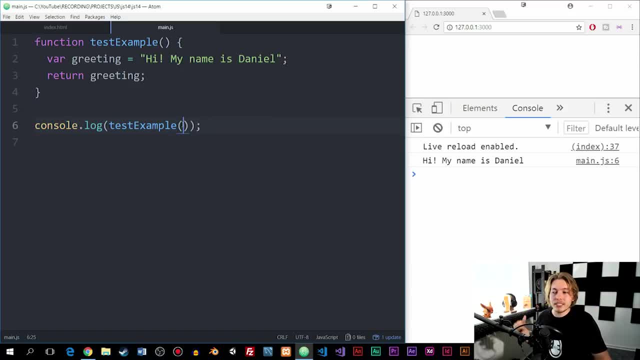 saying that we want to submit an actual name into the function. Now, the way we can do that is using something called an arguments object, which is just a fancy way of saying that we can pass data into the parentheses and send it to the function up here, So inside the function. what I'm going to do is I'm 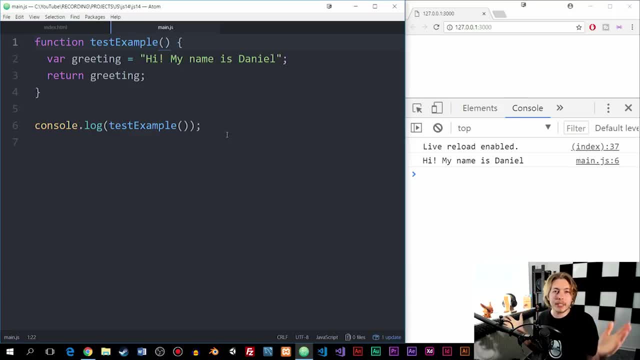 going to create a placeholder. Now, the placeholder can be any sort of name, So I'm just going to go and call it a, And if I want to add more than just one, I can say comma and just say B if I wanted. 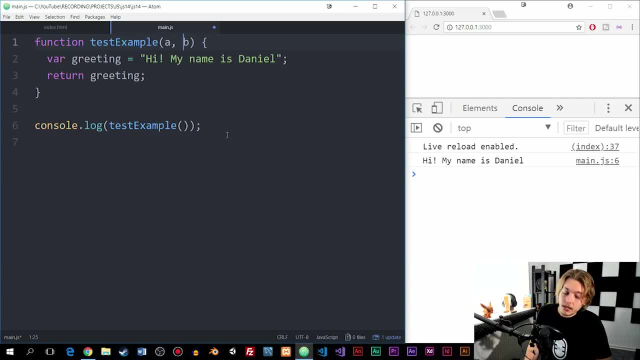 to or space B, doesn't really matter with the spaces, But in this case I'm just going to go and add one piece of data and send it to it. So now we have a placeholder in here And what I can do is I can say: well, when I say, Hi, my name is Daniel, I'm just going to go and delete Daniel and 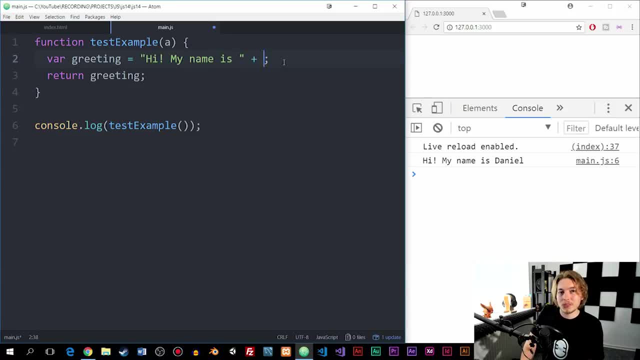 add a string operator, which means that we combine a variable to a string to add one string essentially. So what I can do is I can say I want to add a at the end of it. So down here we do actually console, lock it and call on the function. in here I can go ahead and add a piece. 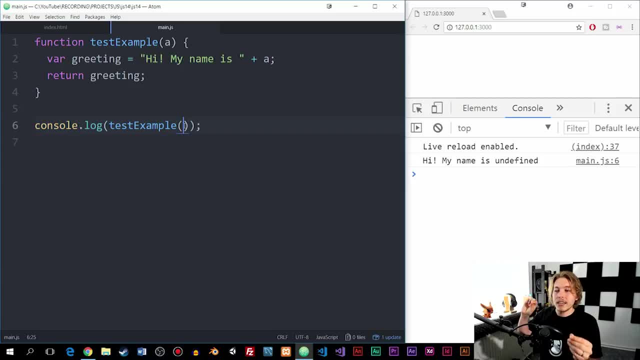 of data into the parentheses in order to send it into the placeholder we called a. So what I can do is I can say double quotes and then I can say: right now you guys can see down here in the console, this is how my name is undefined, because we haven't defined a yet. 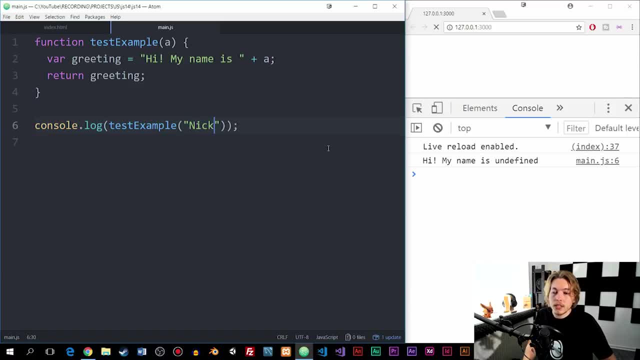 So what I can do is I can say Nick if I wanted to, and now it's going to say Hi, my name is Nick inside the browser here, So this is one way we can do it Now, just to clear something up that you. 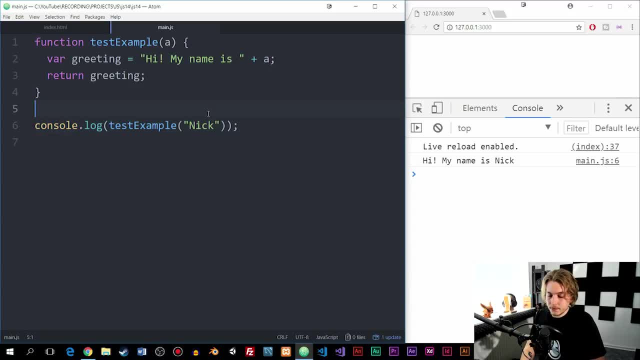 might get confused about later. if I were to go on top of here and create a variable called name, set it equal To Daniel, just to create the other name again and then use the variable name inside the parentheses down here. do notice that it does still work. If I go inside, the console still says: 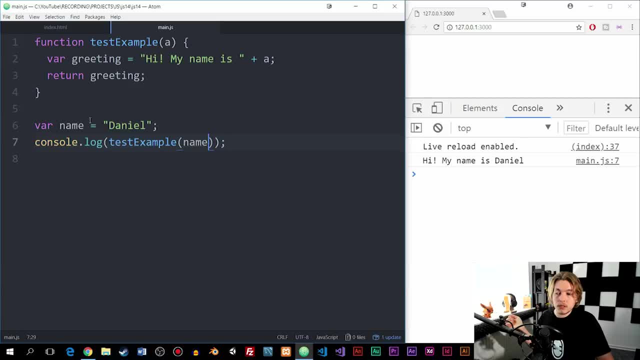 Hi, my name is Daniel, because variable name is equal to Daniel And we use variable name inside the function down here, which is just to show you that the a appears a placeholder. it doesn't have to match with whatever's inside the parentheses down here, So you can still use different name. 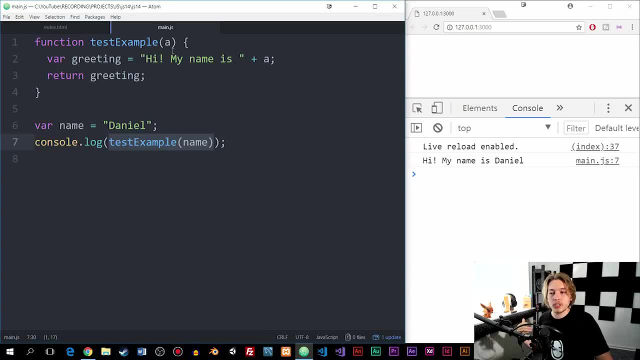 variables inside When you call on it down here doesn't have to match up with what it was up here. Now, the next function I want to talk about is something called an anonymous function, which is slightly different than a name function. Now, an anonymous function is something we usually trigger by either tying 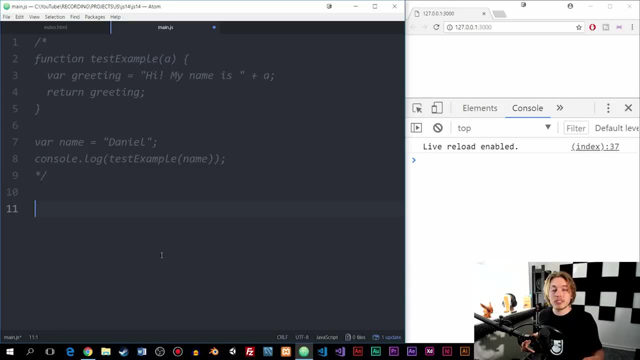 it to a variable or something called an event. Now, events is not something we've talked about yet, But it is something I'm going to teach you later in this course, since it's pretty essential to know about events if you want to do anything with JavaScript whenever the user interacts with. 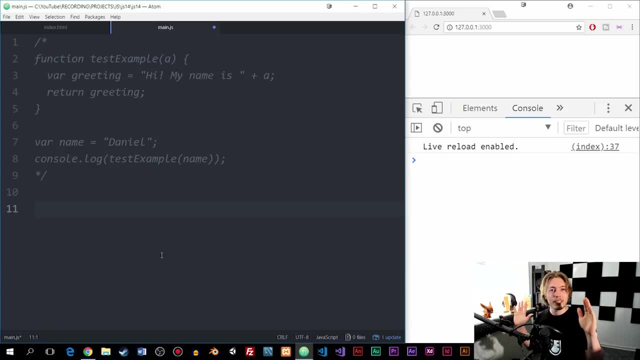 a website. So events is, I'm going to call it an event And I'm going to call it a function. Events is pretty essential, but we're not going to talk about it yet. Now, when I want to create one of these anonymous functions, I can do it by, like I said, tying it to a variable. So what I 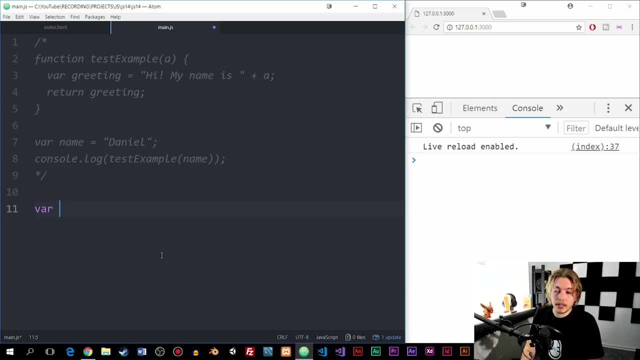 can do is I can create a variable that I can give some kind of name. I'm just going to use the same name as the previous function in the previous example, So I'm going to say test example, then I'm going to set it equal to a function And because this function is anonymous, 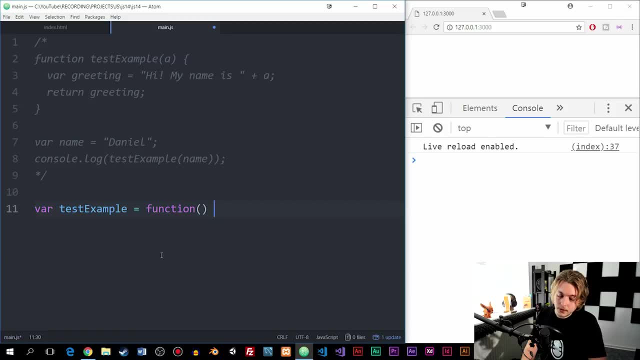 we don't give it a name, So instead we just say parentheses- curly bracket, and then we can just create the same code inside the curly brackets if I wanted to. so I'm just gonna go ahead and paste it in now if I want to call in. 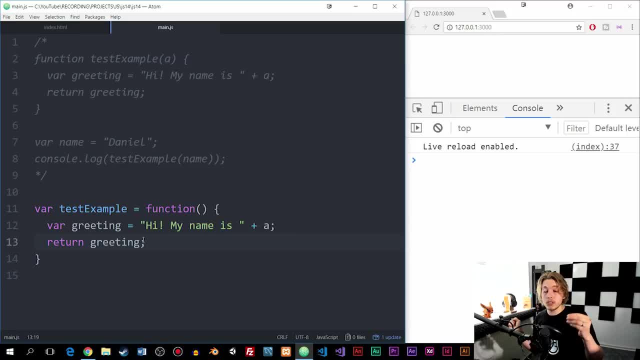 this function. here, like I said, we can do it using events or we can do it using by just calling on the variable. so what I can do is below here I can go and refer to the variable. so I'm gonna say test example, then I'm going to just 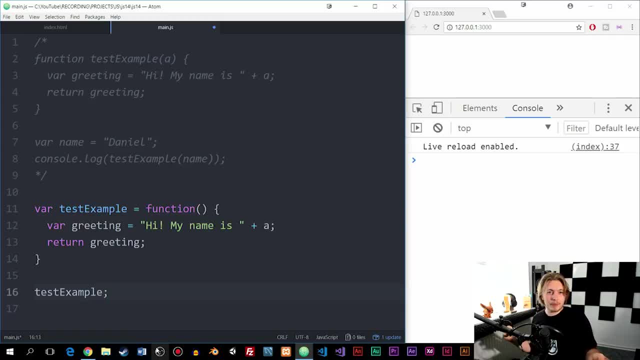 close it off here now. it's not going to work just quite yet, because when we have a function tied to a variable which is anonymous function, the way that we activate the function inside the variable is by creating a pair parentheses right behind the variable name. so this is similar to what we did. 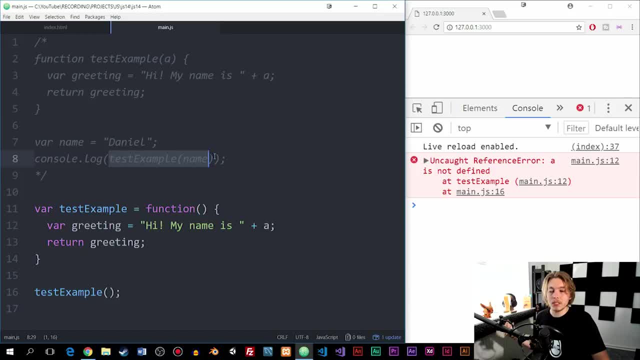 up here. in fact, we just simply called on the function name and then the parentheses, so you know. you might be asking: well, what is the difference here? and I will get to that in just a second. so what I'm going to do is right now, we didn't actually pass in a, a parameter, so I'm just gonna delete that and write. 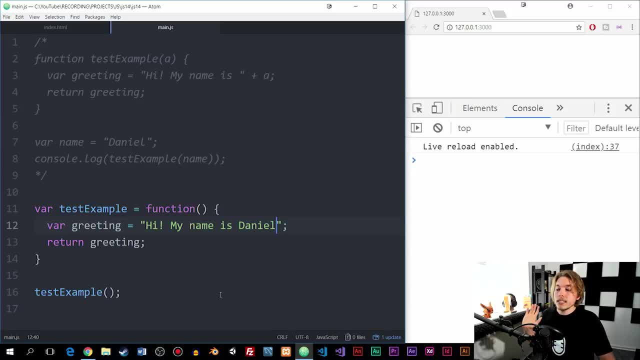 Daniel instead, so we don't get the error message in here now. we haven't actually console logged it yet, so we need to do that as well, because what we did is we actually returned a result inside greeting. so I can actually console dot log parentheses. there we go and save it, and the same way as we would before if I wanted to pass. 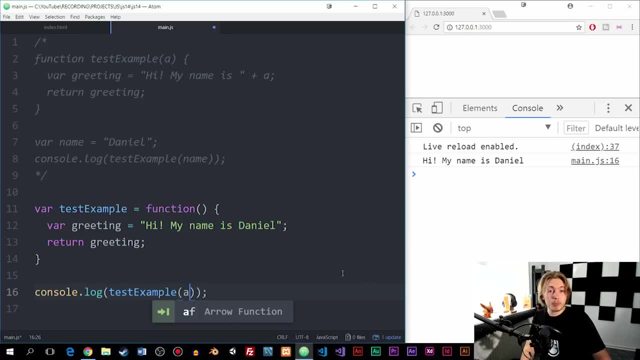 in any sort of parameters. I just do it by including it inside the parentheses here and then inside the function and then inside the actual place down here, so we could say that's it, and then I can actually save it, and then I can actually soft power it up to write the name it. it's actually just just usual by chatting. 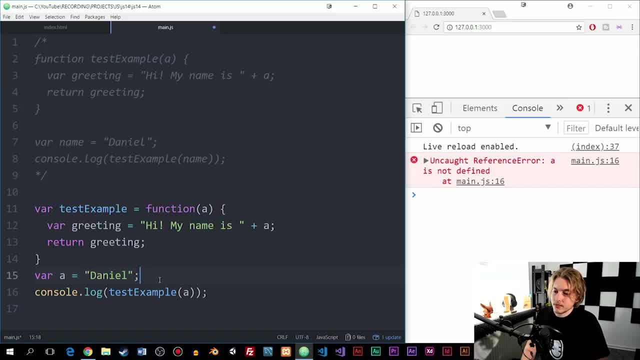 time here: text rondond dot log I. and then back. now we're going to assign the name function to Daniel here and you can just save it. so we can say for example: this time we're going to write A, so you can say: variable A is equal to Daniel. 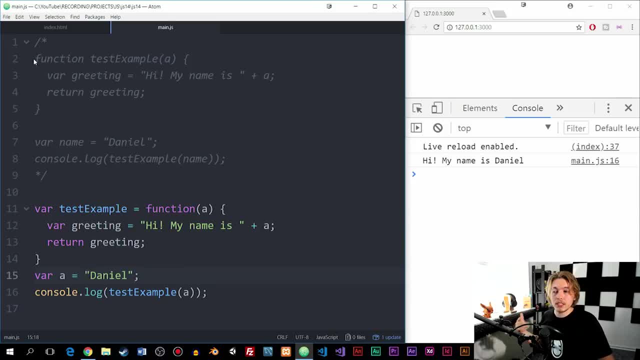 there we go, and now we like to get the result inside the function here. so this is how we can create an anonymous function. now: the difference between an top level inside our JavaScript code, which means that we can use the function whenever we want to inside the code, whereas an anonymous function is hoisted in a slightly different way. Now we 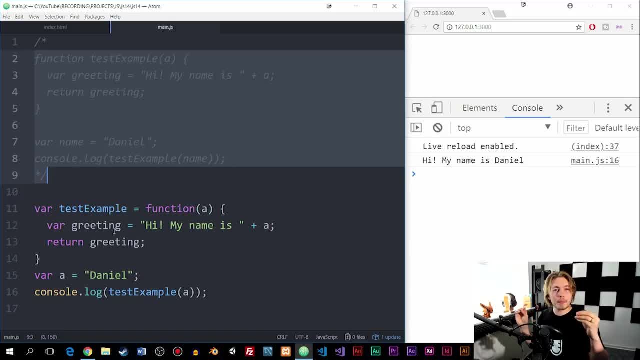 haven't talked about this yet and we will in actually not that many episodes, but we're going to talk about something called scopes and something about hoisting. When we create a variable, the code doesn't actually see the code in the exact same way as we wrote it inside the function. Again, I 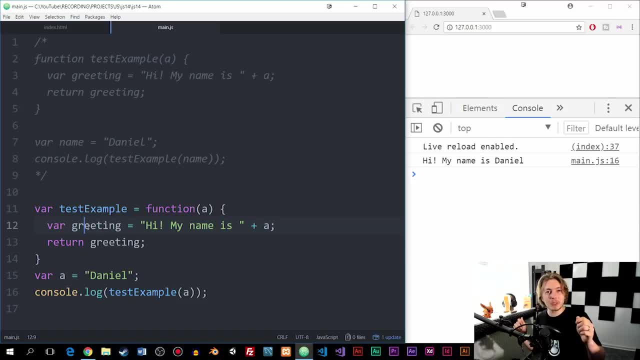 don't want to get off as sidetracking. I'm sort of scared that this is going to confuse too many of you. so we're not going to talk about hoisting just quite yet. We will in a few episodes from now. Then we'll get some very simple examples to illustrate what exactly hoisting is. but the basic. 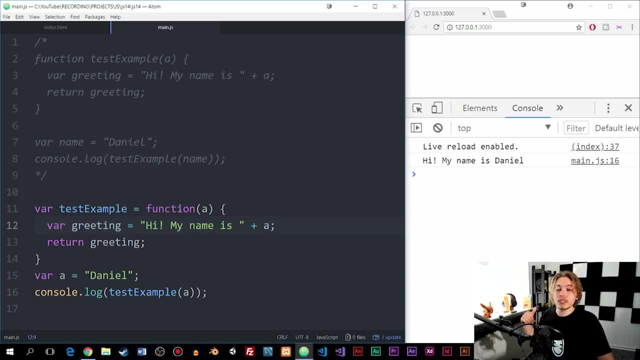 idea here is that when we create an anonymous function because it's equal to a variable, the variable gets stored at the top level in the same way as the function does, but we don't actually have the value from the function yet Until we actually get to it down in the script. So that's the basic difference between anonymous and 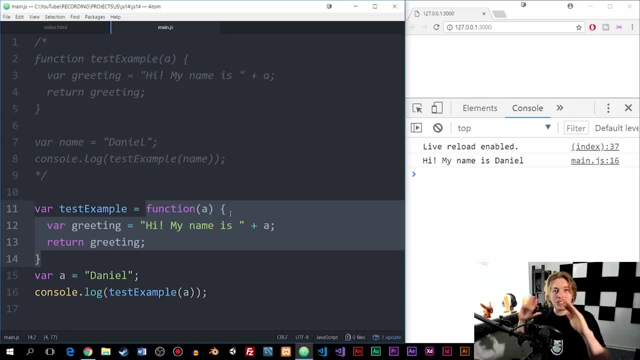 named functions. Again, if I just confused you, just forget about everything I said. We'll get to it once. we do actually get to talk about hoisting, and later we will actually talk more about anonymous functions. So next example: Now we also have something called an immediately invoked functional. 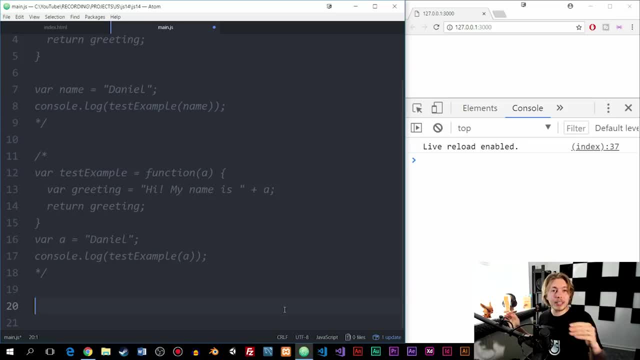 expression. and this is basically a function that, again, like the anonymous one, doesn't have a name, but it's a function that can be done as soon as the code gets loaded inside the browser. So if I were to create a function here just by creating function parentheses, curly brackets, then I can. 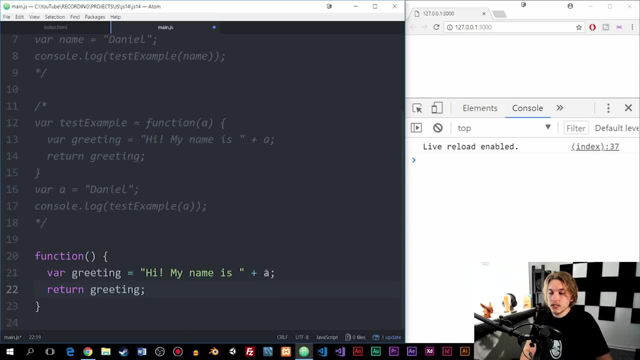 create some kind of code here, like what we did up here, But instead I would like to just console log this inside the actual console. So I'm going to say, Daniel, and I'm just going to go ahead and console log it instead of returning it like we did down here in the code. 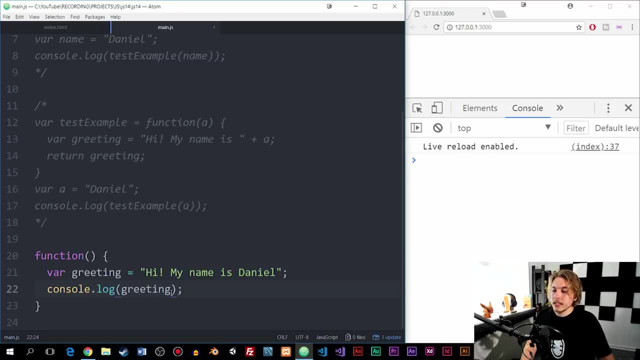 log greeting. Now, as you can see, we get a uncut syntax error. If I want this blogger code to run immediately inside the browser, we do need to do a couple of things to make it into a immediately invoked functional expression. So what we need to do is, first of all, we need to wrap this entire 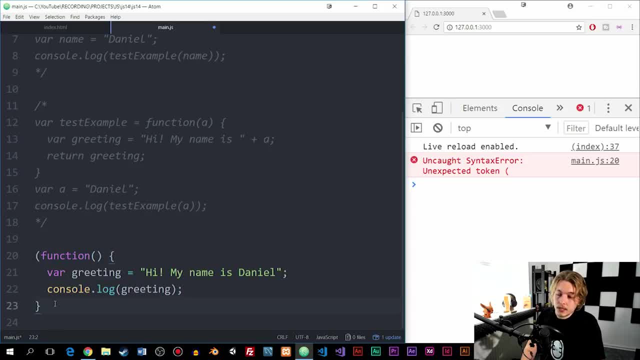 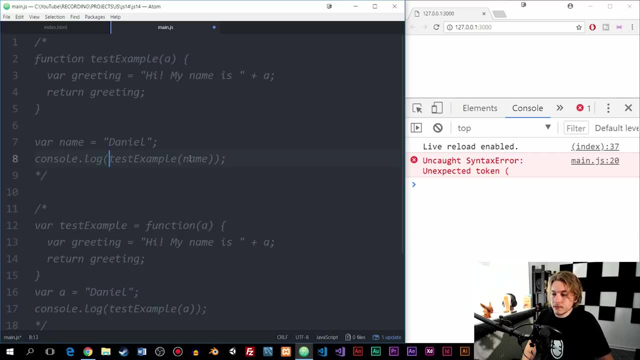 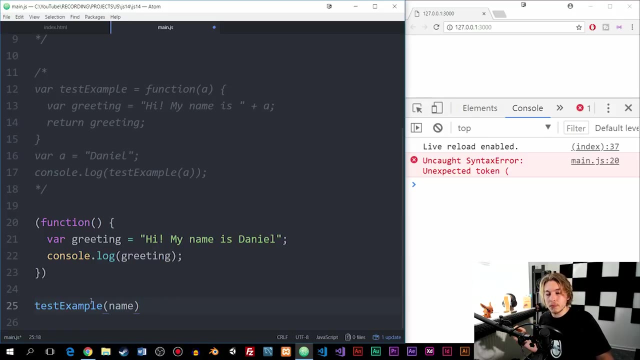 function inside a pair of parentheses And then afterwards what we need to do, in the same way as when we would call out a function by this example here. I'm just going to bring it down So we can see it. When I want to call the test example function, we then say test example and then add the. 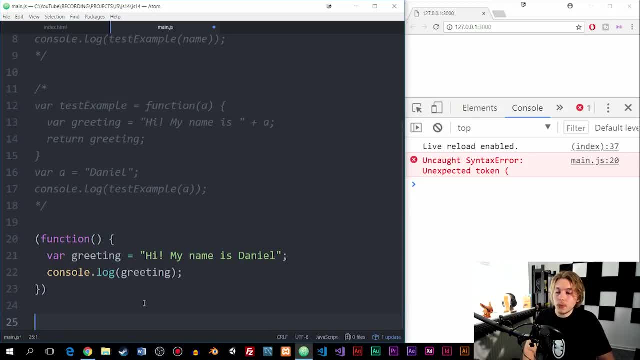 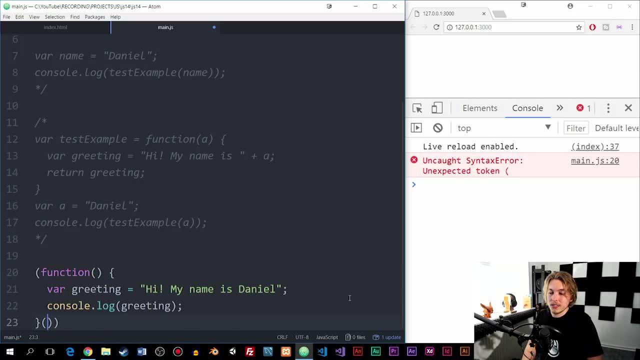 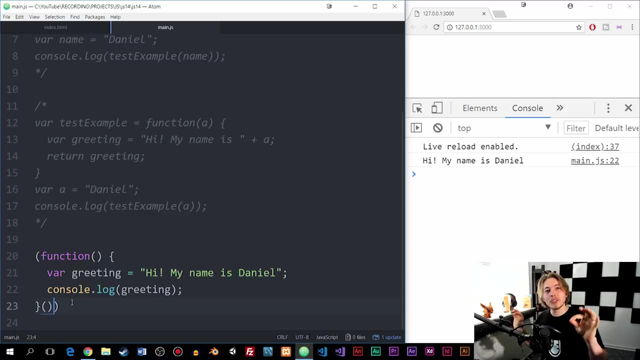 parentheses at the end here. So in the same way, if I want to call this function immediately, need to add a pair of parentheses right after the function, if that makes sense. So we're going to add it right before the closing parentheses. that was wrapped around the entire function. So in this example here, make sure you put the. 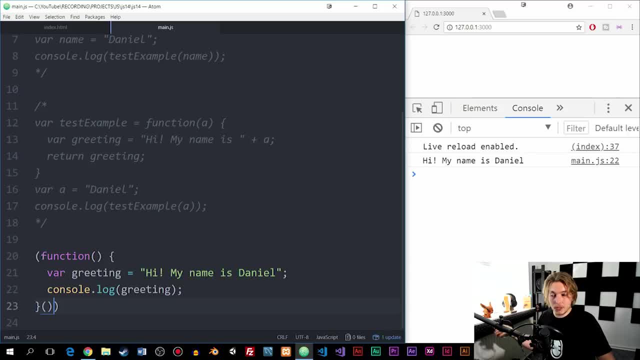 parentheses in the right place. We have an opening parentheses, the function with the curly brackets, then a opening and closing parentheses and then the closing parentheses. that belongs to the first opening one. Okay, so when we do this, as you can see, it's going to run. 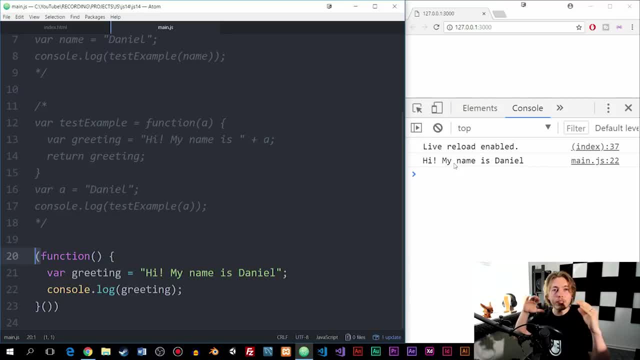 the code immediately as the document gets loaded inside the browser And, as you can see, inside the console. we do have Hi. my name is Daniel, So these are functions, And what we're going to focus on, at least in the beginning, are just named functions, which is the first example we did, which is pretty. 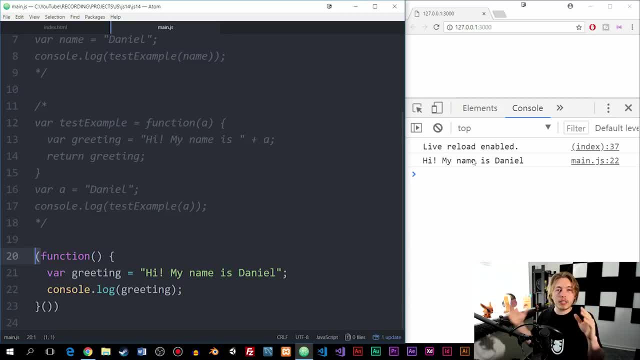 simple to do, to use And once we have done a couple of examples in a couple of exercise files, probably in the next episode we'll get to actually experiment a little bit with these functions and see how we can use them inside our JavaScript code in order to do something with the data that we have inside our website. So I hope you guys. 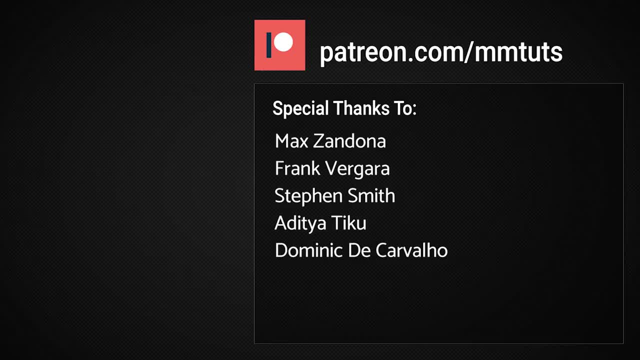 enjoyed. I'll see you next time. Thanks for watching.